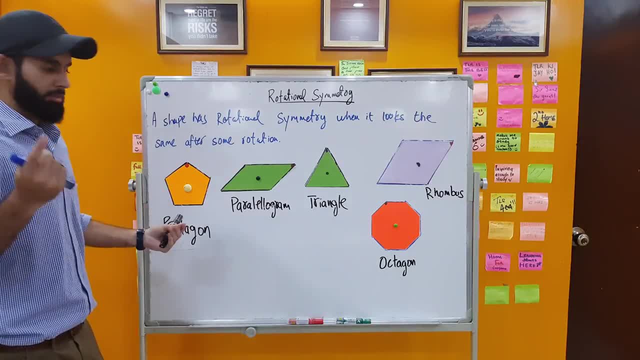 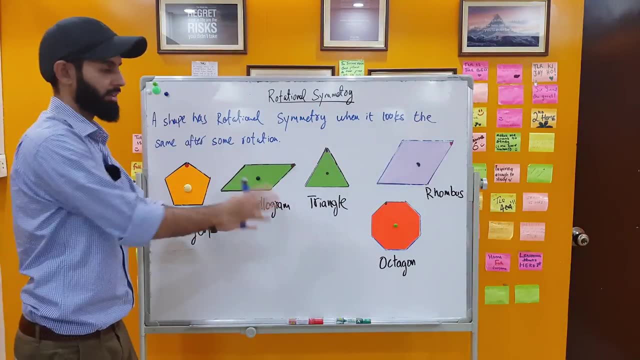 times we get the exact same shape right. And, by the way, bear in mind that this pentagon, this triangle, this octagon, they're all regular polygons in the sense I mean the ones that I've made here, in the sense that all the five sides of this pentagon are equal. 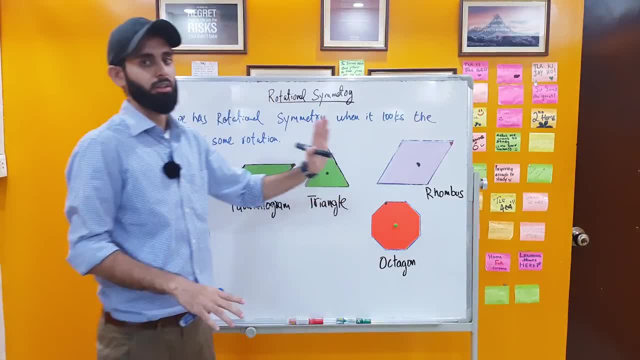 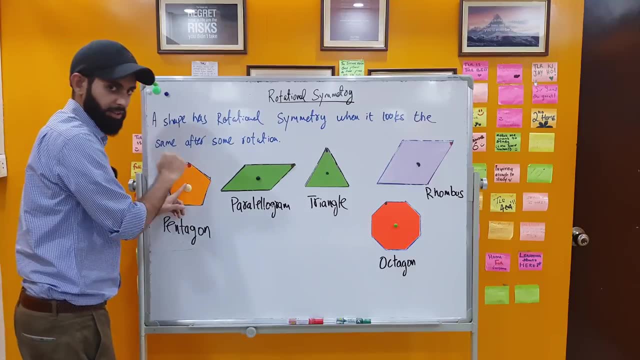 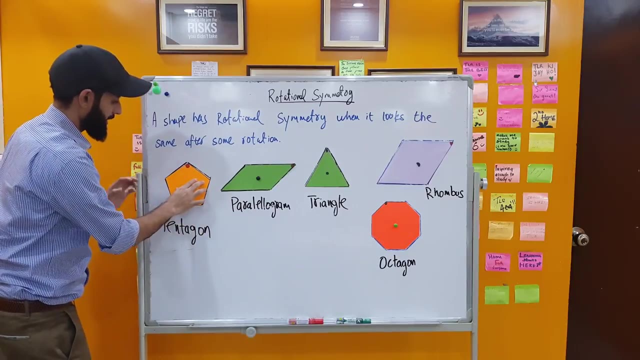 All the three sides of this triangle are equal, and all the eight sides of this octagon are equal, right? So let's get started. So I've marked a red spot here for reference, which means that I'll stop when this point is back at its original place, right? So I'm going to start rotating and 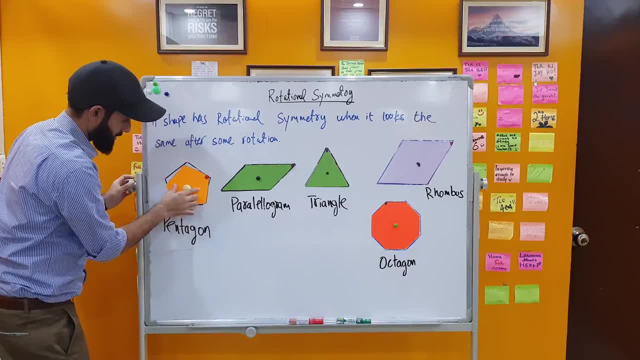 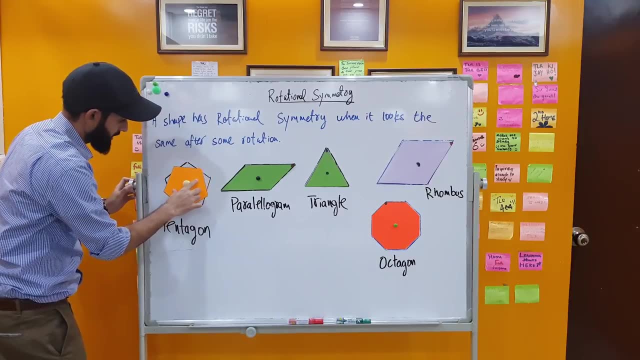 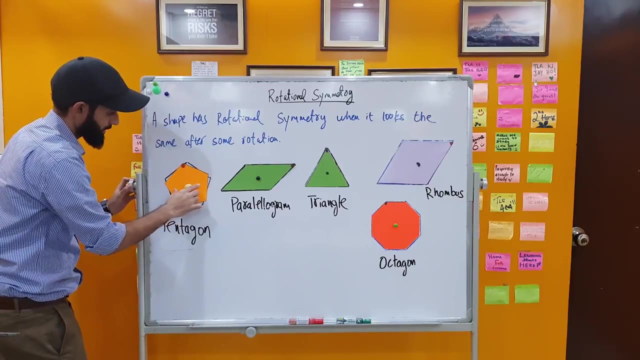 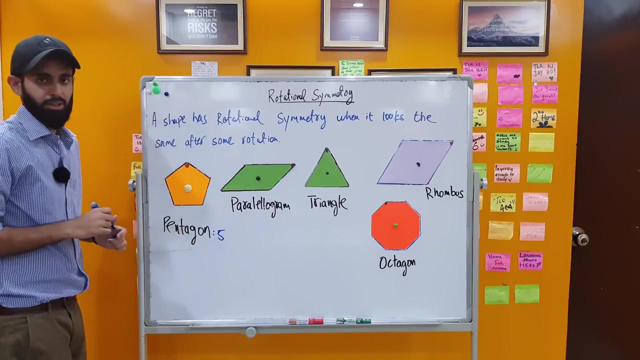 then I want you guys to count with me. So that's once, that this is now twice, twice, four times and then finally five times. So that means a pentagon, a regular pentagon, to be precise, has a rotational symmetry of order five. All right, now let's talk about this parallelogram that I've 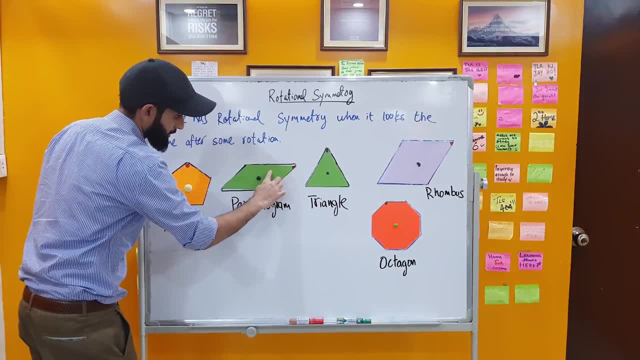 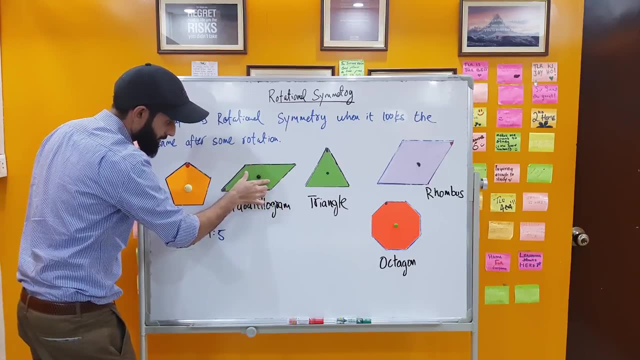 made here Again, this is the fixed point, the through which that I'm going to be rotating it. So no luck there. Let's keep on going, let's keep on going and finally we get the exact same shape. So that's one once. 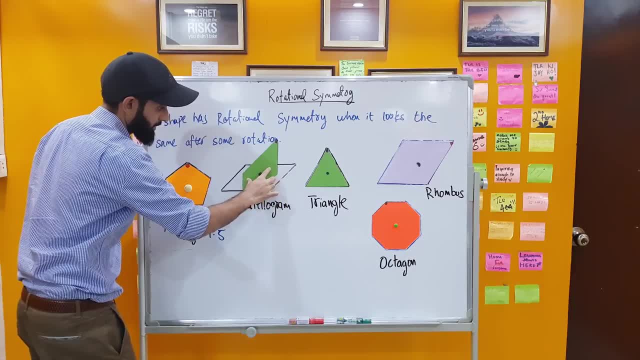 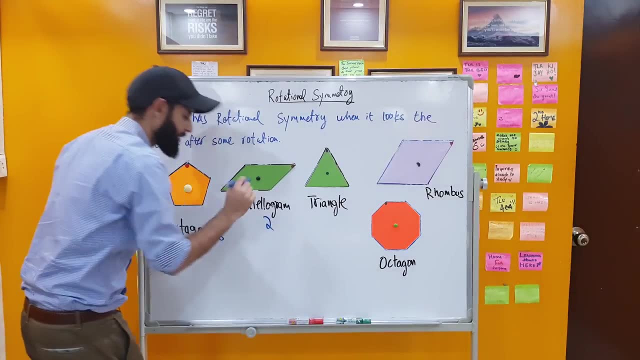 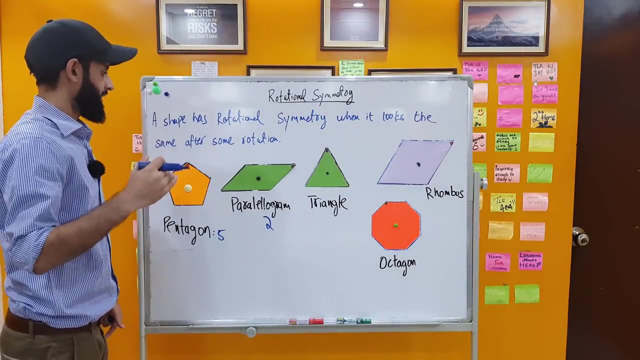 So no luck, Let's do it again. That makes it twice. So that means a parallelogram has rotational symmetry of order two. Now, at this point I'd like to point out that you should also know, after you've figured the order of rotational symmetry, the number of degrees you need to rotate in order to get the exact same shape. 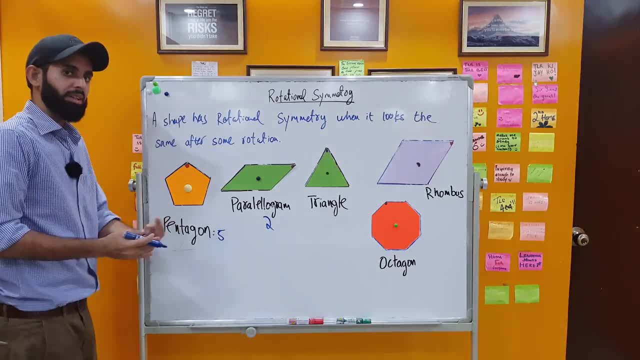 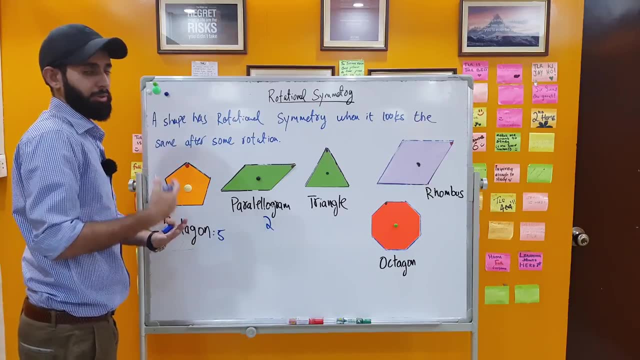 Now there is a very simple formula for that. What you're gonna do is you're gonna take 360 and then divide it by the order of rotation symmetry. So if I want to figure out what, the well. if I want to figure out the number of degrees, I need to rotate a. 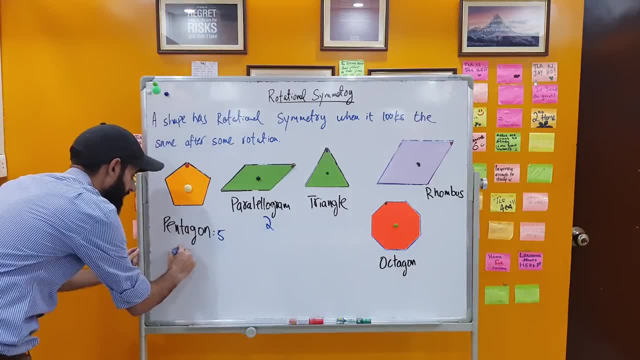 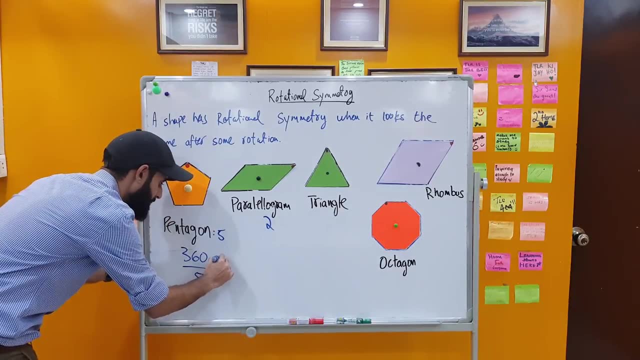 regular pentagon in order to get the exact same shape. so what I'm simply gonna do is I'm gonna take 360 and I'm gonna split it five ways, which is the order of rotation symmetry of a regular pentagon. so that's gonna give me what. 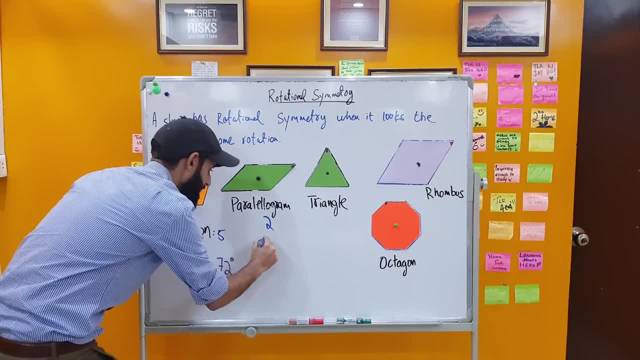 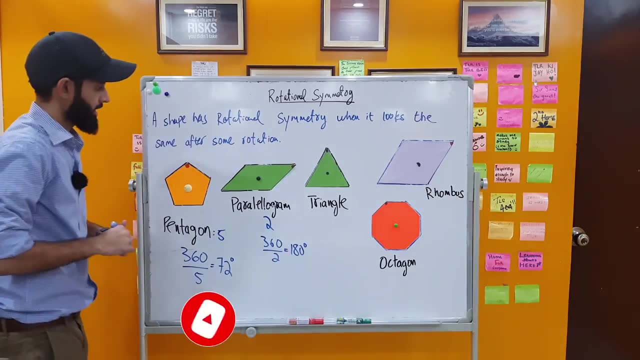 that's gonna give me 72 degrees. right, what about a parallelogram? I'm sure you figured it out before I did: 360 divided by 2 is 180 degrees. now let's move to this triangle, this equilateral triangle that I've made here. now, here's my fixed point. 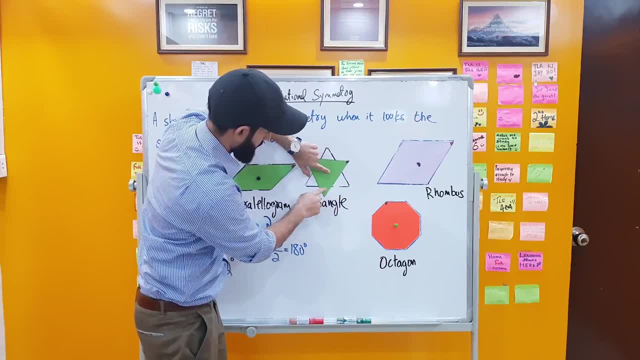 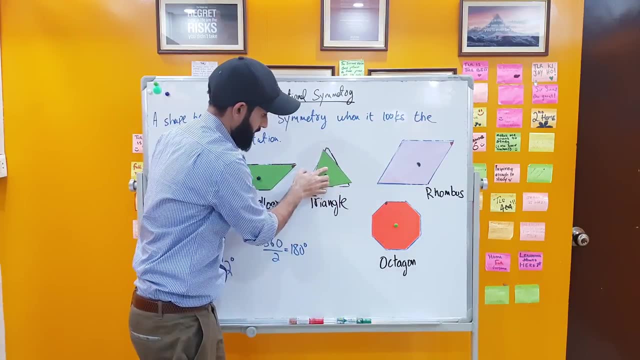 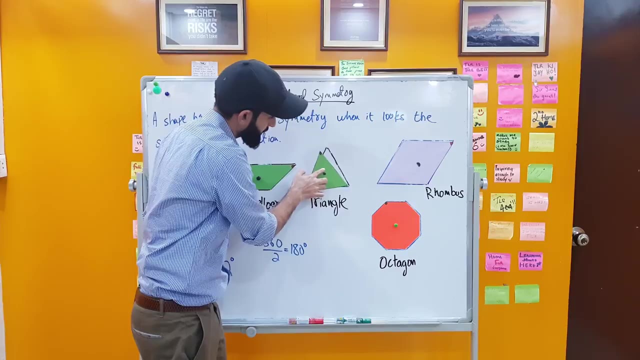 right, so I'm gonna rotate it from here. and so that's once right, let's do that again. that's twice. I need to get this red spot back to its original place, so let's do that one more time. so that makes it thrice. so that means I got the. 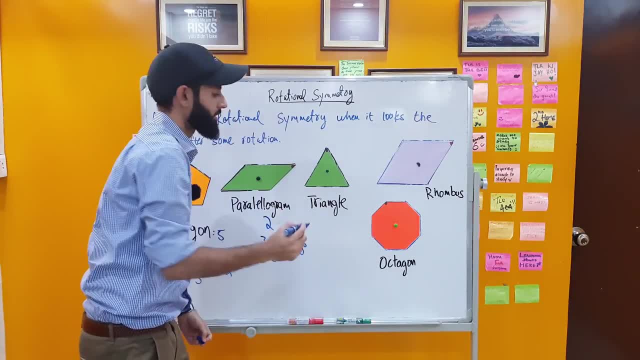 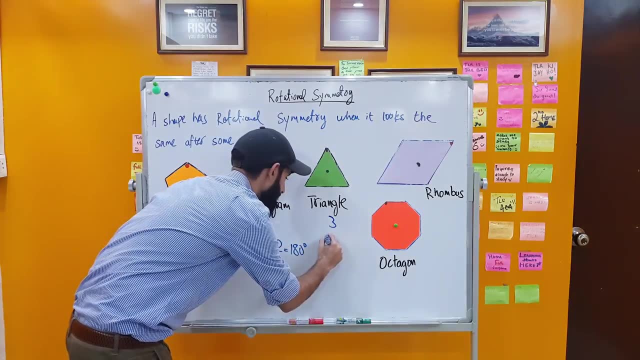 exact same shape three times, so a triangle, or an equilateral triangle to be precise. as order of rotational symmetry, 3 and again, if you want to figure out the number of degrees you need to rotate. so that's gonna be 360 divided by 3, which. 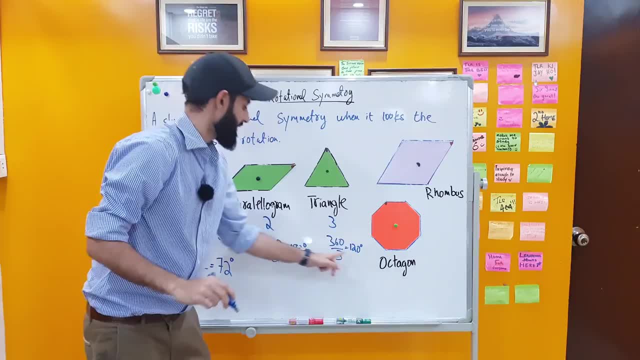 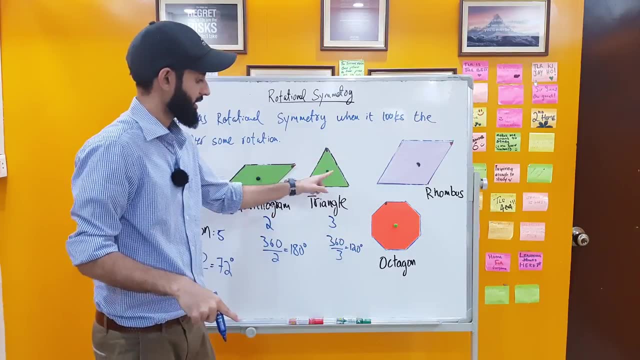 is equal to 120 degrees. now this 120 degrees, I should point out, is from the center right. so from the center, if you rotate this triangle 120 degrees, you get the exact same shape right. so let's talk about this rhombus here again. here's my 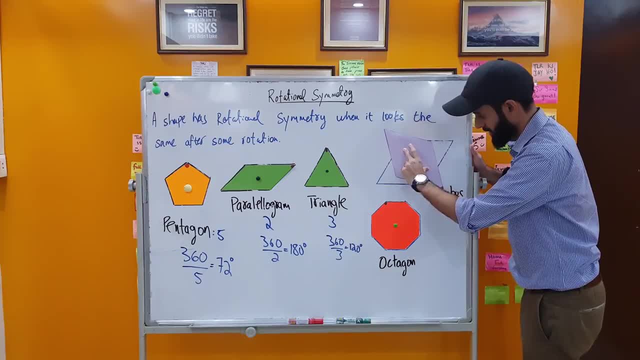 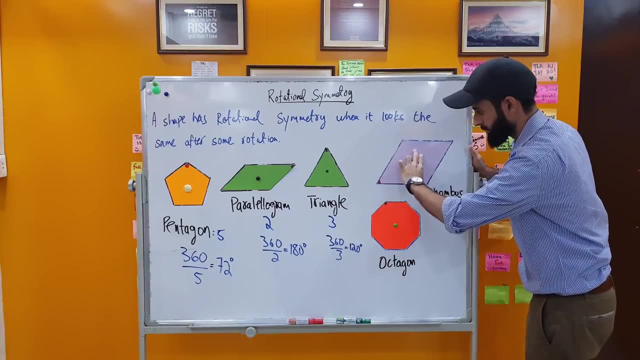 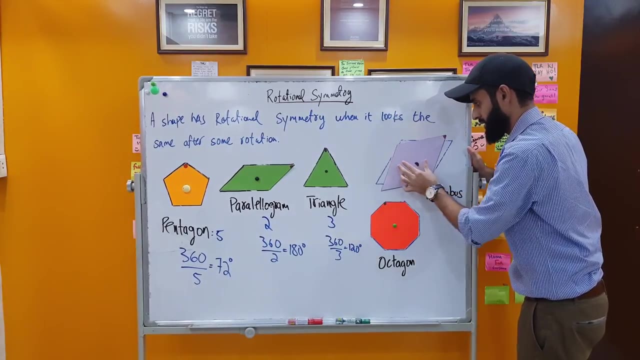 fixed point. so that's a quarter turn. no luck there. so that's half a turn. half a turn basically means 180 degrees. so I got the exact same shape. so that's once. let's do that again. and that makes it 2. so that means a rhombus has rotation symmetry of order. 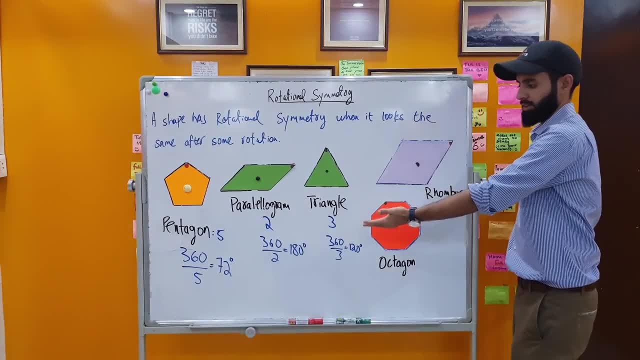 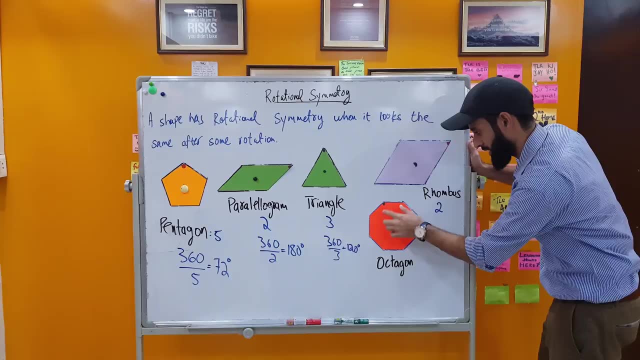 2, same as a parallelogram, right and again, the angle that you must rotate is going to be the same, which is 180 degrees. now here's an octagon. I want to give you a hand here. so again, remember, i need to get this red spot back to its original place. so that makes it once. 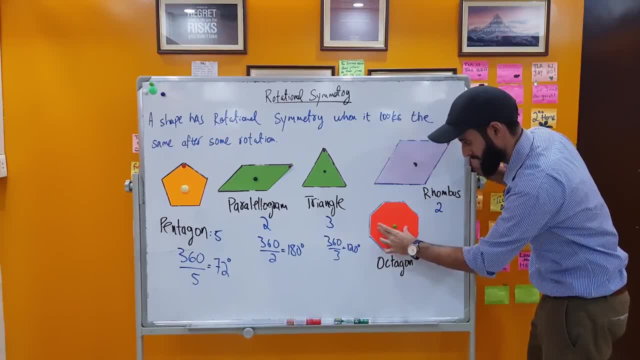 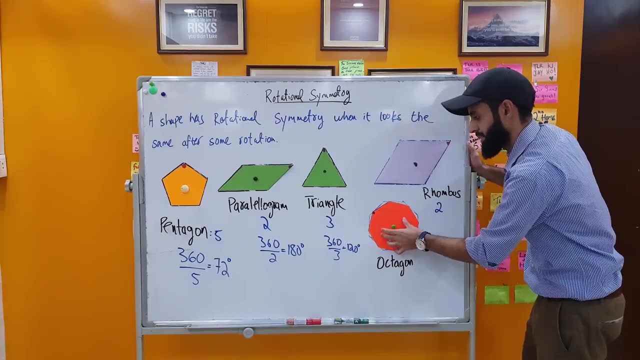 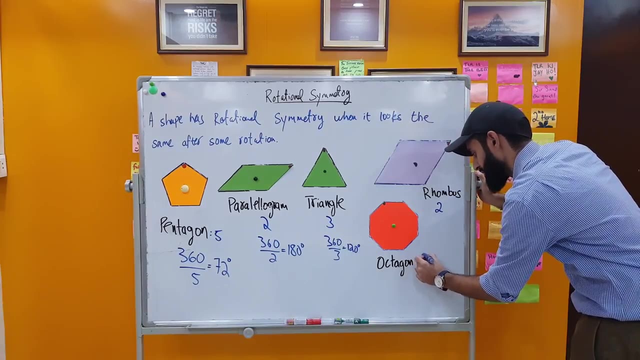 twice, three times, four times, five times, six times, seven times and then finally eight times, right? i'm sure you figured that out before i did so. an octagon has order of rotational symmetry, eight and again. if you want to figure it out, if you want to figure out the number of degrees that 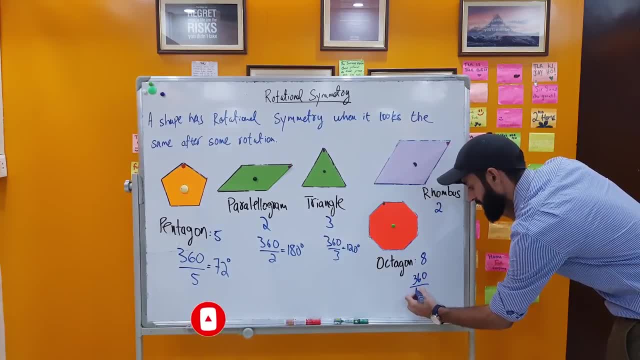 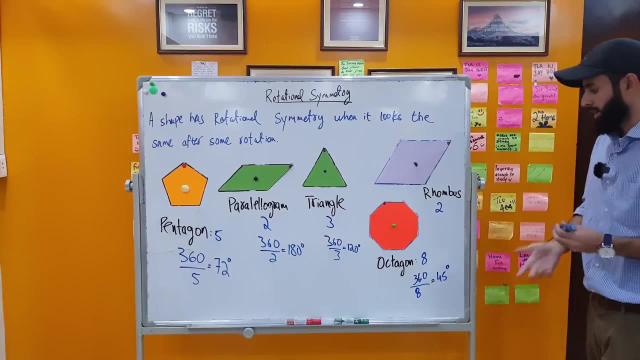 you must rotate, so for that i'm going to do 360 divided by 4 or 360 divided by 8, sorry. so that's going to be equal to what? uh, 45 is it? yeah, that's 45.. anyway, so that's all for rotation.